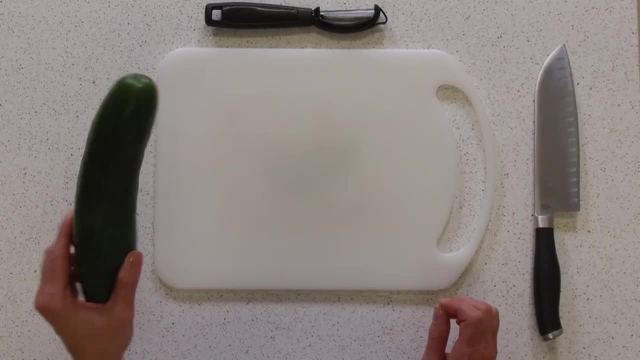 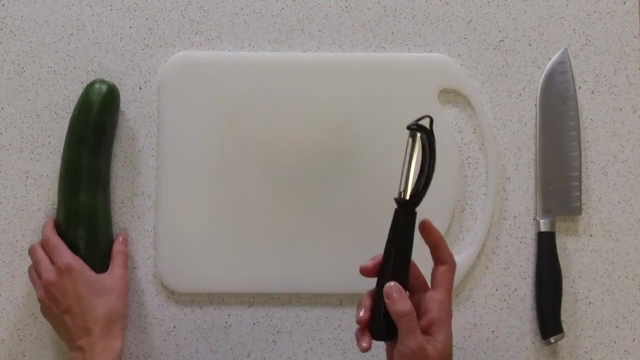 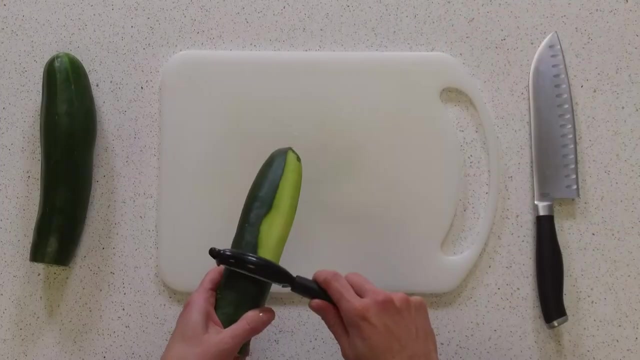 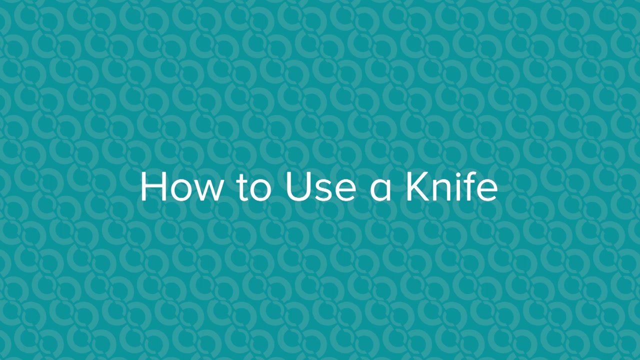 before chopping or cutting: You can peel the produce or you can eat it without peeling. If removing the skin of the produce is easiest, to use a peeler. before chopping or cutting, Hold your pointer finger and thumb where the blade meets the handle. 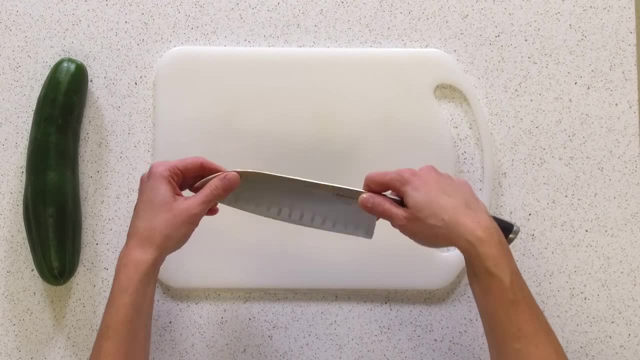 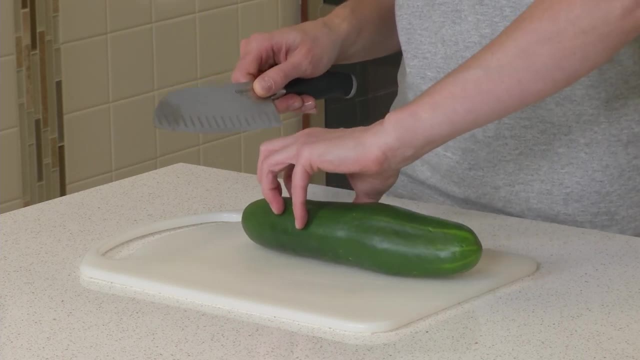 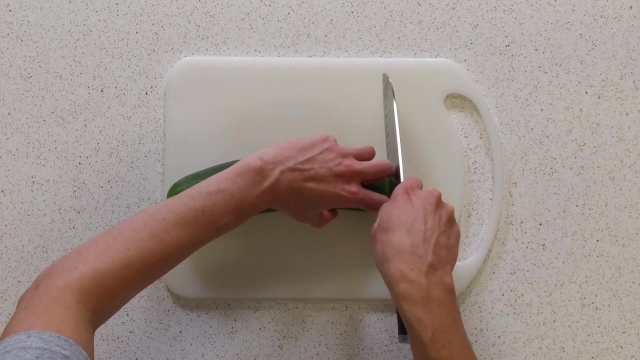 Wrap your fingers around the handle. This will give you better control. Hold your fingers in the shape of a claw to hold the produce. Your fingertips should face away from the sharp edge of the knife. Your knuckles may touch the top, dull part of the knife. 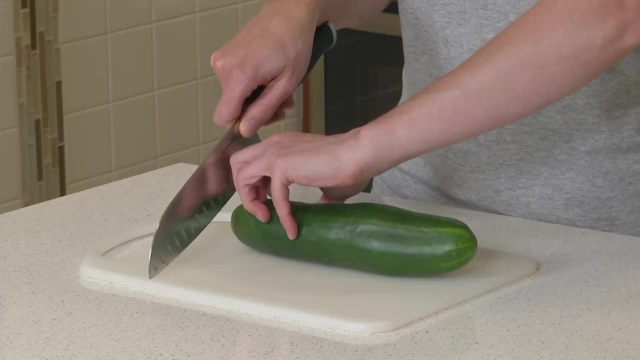 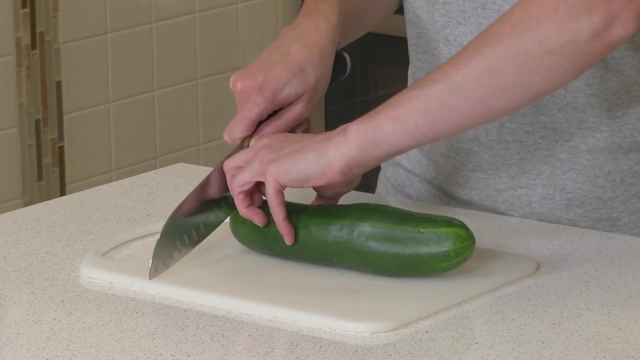 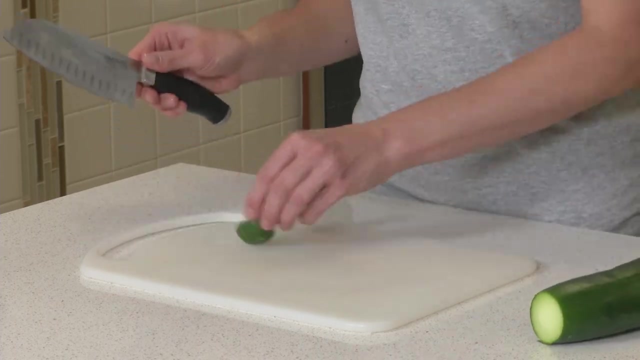 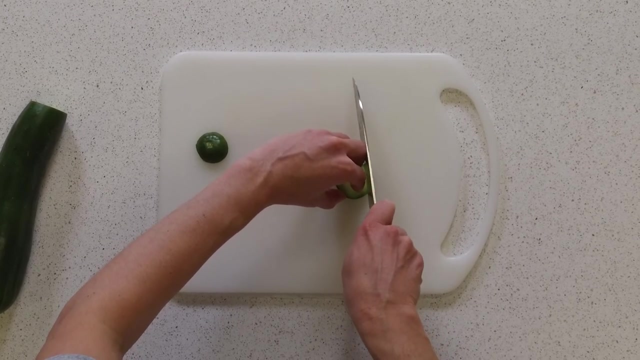 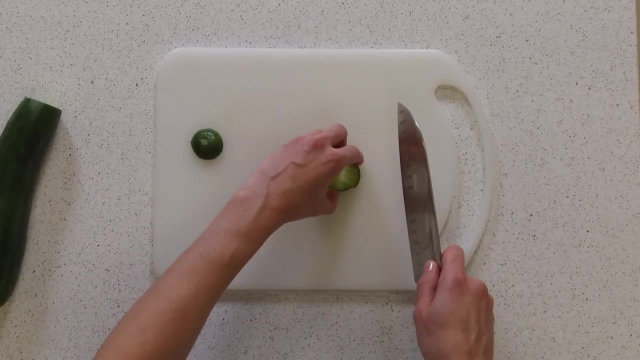 to help guide your cutting, The tip of your knife can rest on the cutting board. to help with the control, Cut straight through the produce. Using the same technique, cut the cucumber into strips, Turn the vegetable strips 90 degrees and cut into smaller cubes. 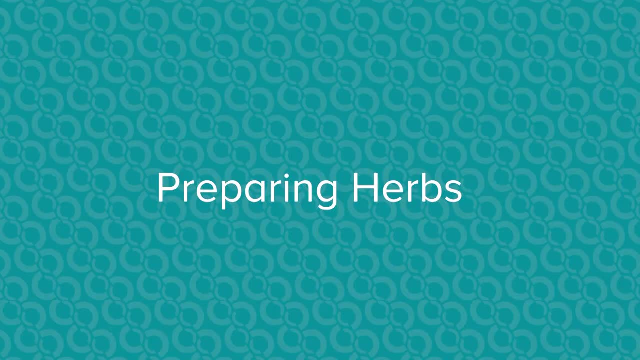 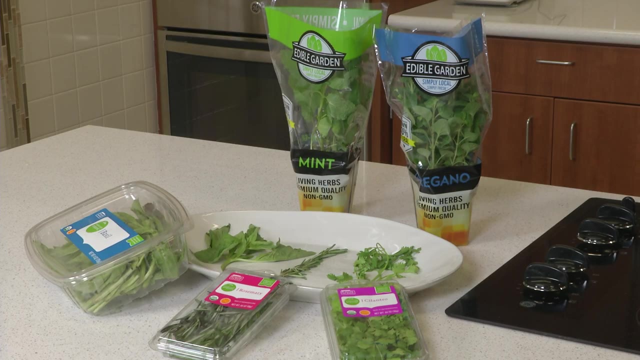 Use a knife to cut the cucumber into strips. Use a knife to cut the cucumber into strips. Use a knife to cut the cucumber into strips. Now here is how to cut herbs for added flavor to your meals. Here are a few examples of herbs. 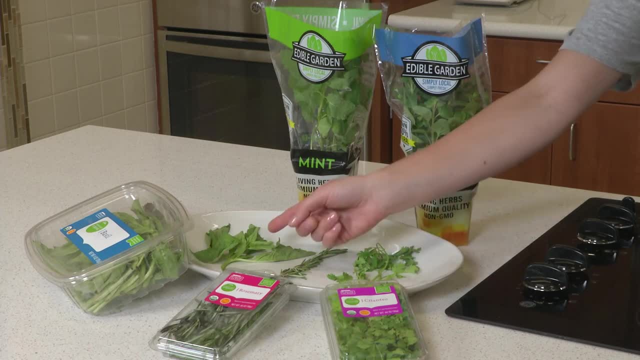 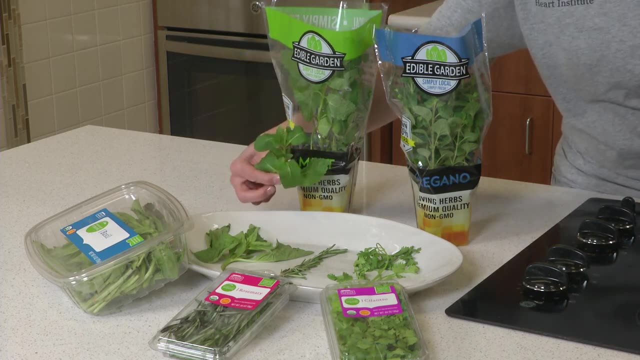 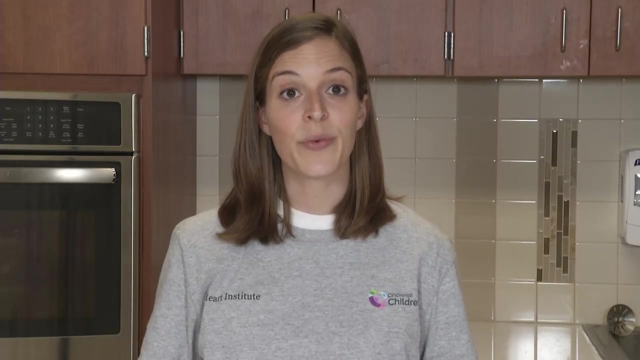 Cilantro, rosemary, basil, oregano and mint. Today, we'll be using basil. All herbs can be cut the same way. All herbs can be cut the same way. Herbs can be sliced thin or chopped. 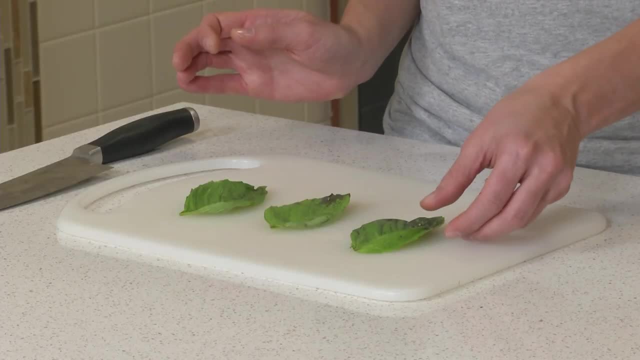 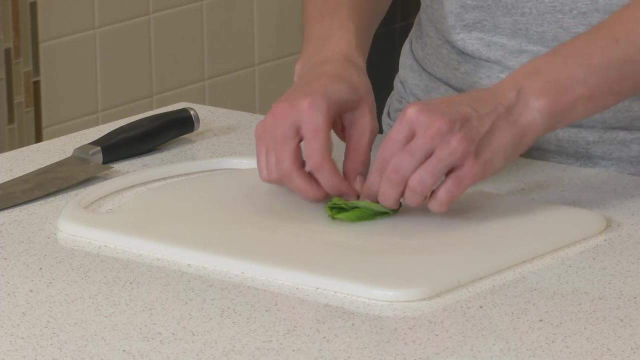 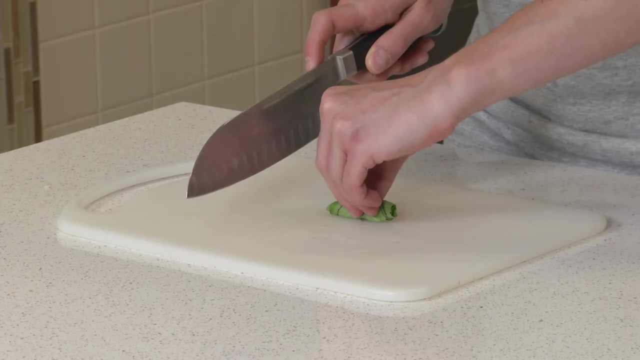 For thin sliced leaves: stack leaves on top of one another. For thin sliced leaves: stack leaves on top of one another. Then roll the leaves tightly. Hold the roll in one hand. Remember to curl your fingers in the shape of a claw.